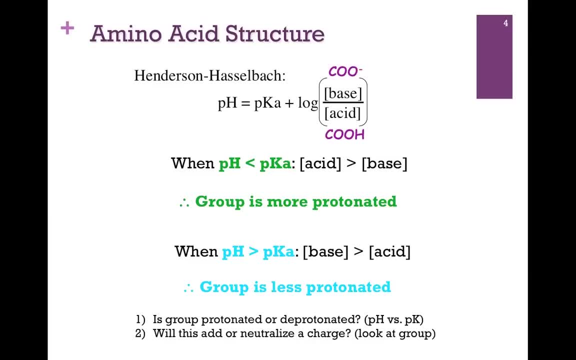 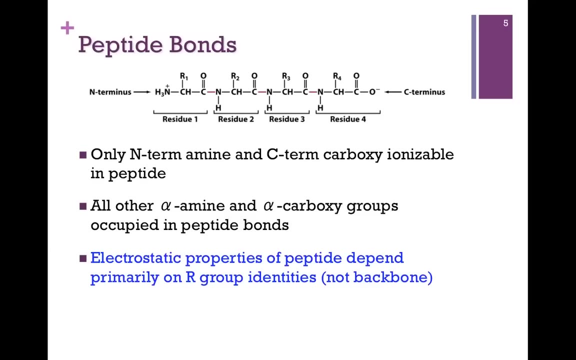 If it were more deprotonated it would be neutral. So again, first look at this general rule- pH versus pK- that always applies- And then look at the group to know: by protonating it, am I adding a charge or am I neutralizing a charge? We find that when we string together, 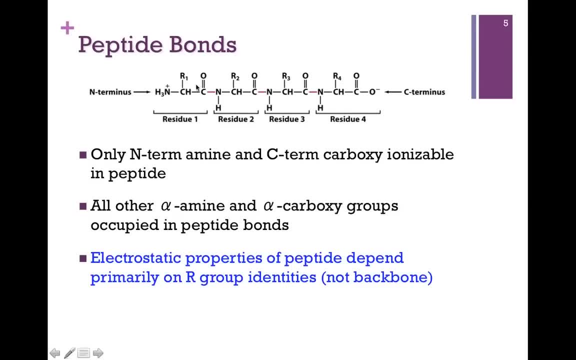 these amino acids to form a peptide. we're joining those ionizable alpha carboxy and alpha amine groups to form those peptide bonds so they're no longer ionizable. The only groups in our backbone that are ionizable are the alpha amine group on our 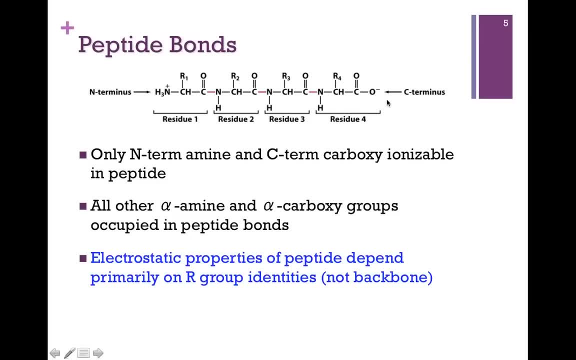 first residue and the alpha carboxy group. on our last residue, You'll notice that physiological pH, we have a plus one charge on the amine group and a minus one on the carboxyl group, and so it nets to zero, Therefore, the electrostatic properties of the molecule. 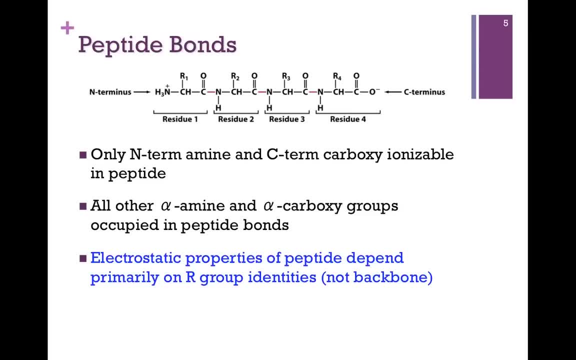 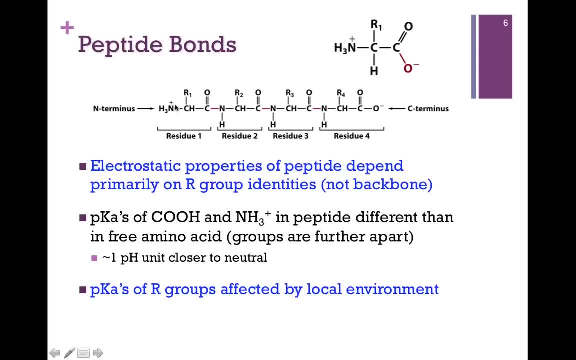 have more to do with the nature of those side chains and their ionizability. One thing I would point out- and I'm not going to go into too much detail on this, but I'm going to point out- is that the pKs for those end groups, that is, the alpha amine group and alpha carboxy, 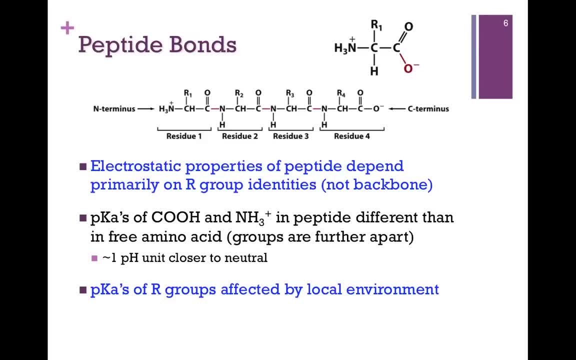 are different in a peptide than they are in the free amino acid. Let me just illustrate what I mean. At the top of the screen we have a single amino acid. You'll notice the alpha carboxy and alpha amine groups are attached to the same carbon atom, very close to one another, and they strongly 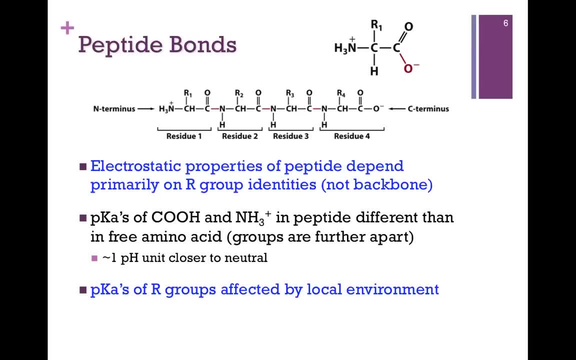 influence each other. This makes the carboxyl group more acidic and the basic group more basic. However, in the peptide group, we have a single amino acid and we have a single amino acid. Notice that they're widely separated from each other, so they have less of an impact on each. 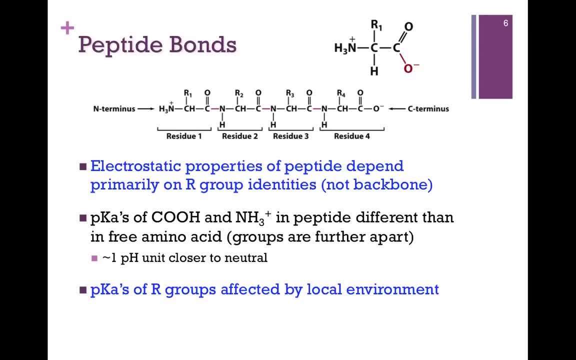 other. This means the carboxyl group is less acidic and the amine group is less basic. This means that they're a pH unit closer to neutral, and the point here is that within a peptide or protein those pK values could be different than they are in the free amino acid The other way. 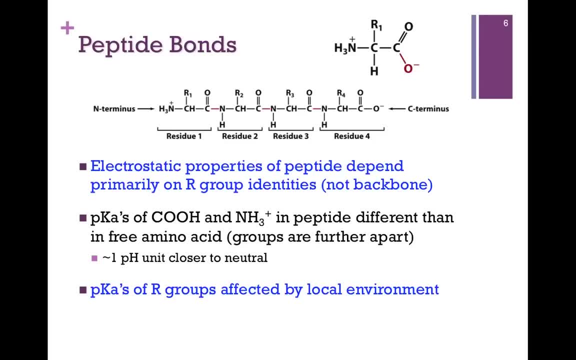 they can change is that the pKs of those side chains can be affected by the carboxyl group. In other words, our protein is going to fold up to a certain conformation and that local environment where that R group is located might influence it to have a higher or lower pK value. 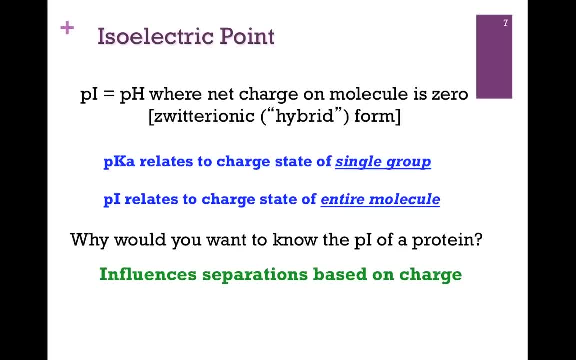 than it would as a free amino acid. So we've looked at this pH versus pK and the charge state of an individual group. but what about the charge on the overall molecule? For that we want to look at the isoelectric point, or PI. The charge state of an individual group is the charge state of an 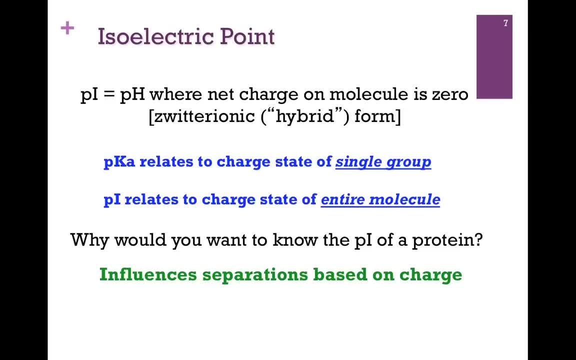 entire molecule. This is the pH, where the net charge on the molecule is zero. This is the isoeuteryonic form. Remember, if we're looking at pH versus pK, if pH is equal to pK, it's half in one. 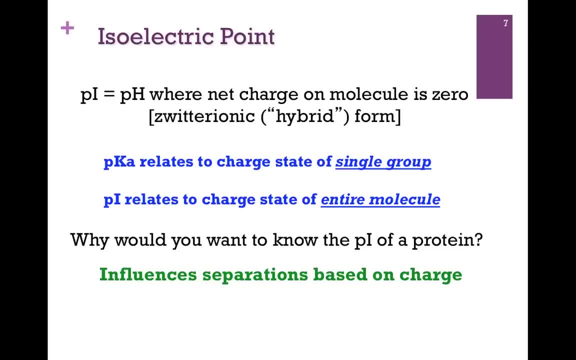 form and half in the other. So in this case, for the overall molecule, if pH equals PI, the net charge is zero. So remember, the pK relates to the charge state of a single group, The PI relates to the charge state of the entire molecule. 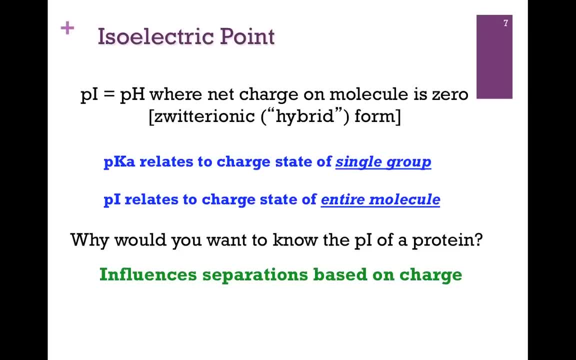 So the question is: why do you need to know the PI of a protein? Well, remember, if the pH is equal to the PI, the net charge is zero. If we want our protein to carry a net charge, we need to be able. 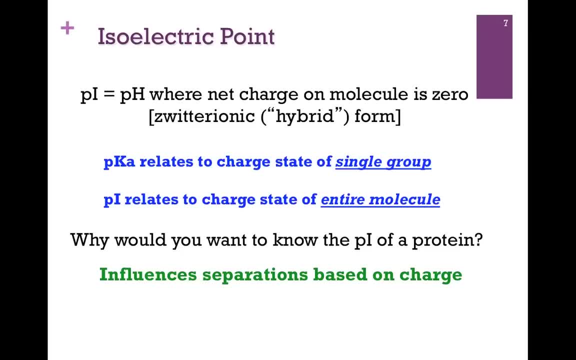 to adjust that pH based on that PI value. Why would we want our protein to carry a net charge? Well, we may be trying to separate our protein based on that charge. We'll see more on this when we get to a later lesson. 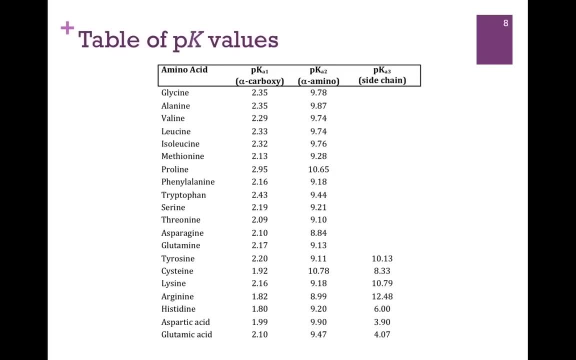 I want to show you here a table of pK values. You'll see this on the exam, and so I want you to know how to interpret it. This is the list of all the 20 common amino acids, and you can see they all. 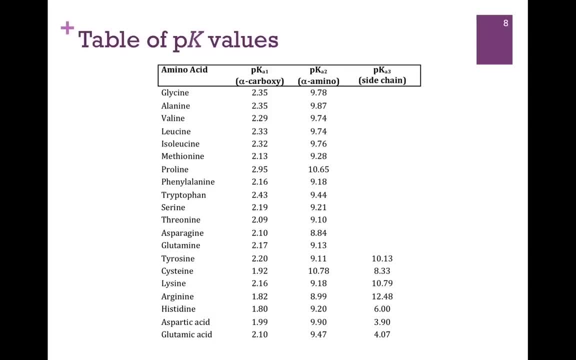 carry a pK1 and pK2 value. The pK1 is the alpha carboxy group and you can see that it hovers around two, so a very acidic group. and pK2 is the alpha amine group, around 9 or 10 in alkaline pH. Notice: 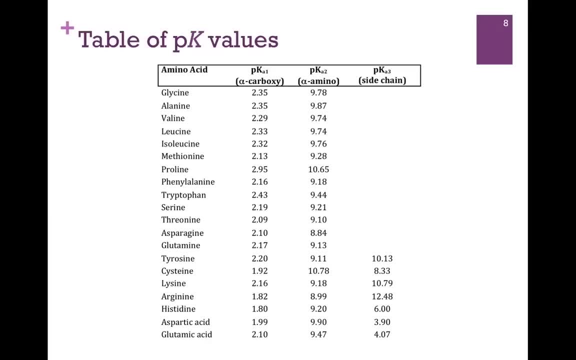 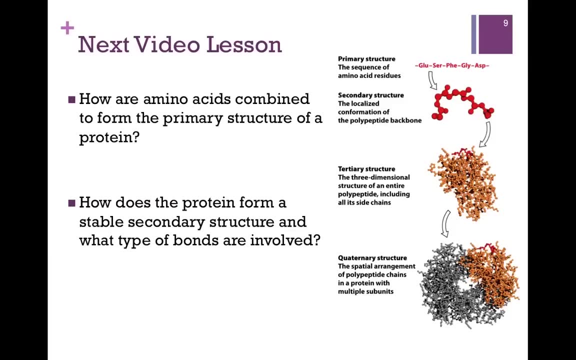 the pK3 for that side chain only if it's an ionizable side chain and it varies depending on the nature of the functional group. In our next lesson we want to look to see how amino acids are combined to form the primary structure of a protein, and then how does that protein form a stable secondary structure. What types of bonds are involved?